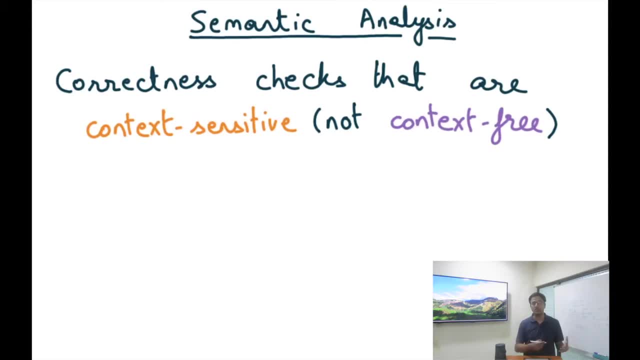 anything that cannot be done in the parsing step and is con and because it was context sensitive, is basically done in the semantic analysis step. all right, So here are some examples of context sensitive analysis. for example, all identifiers in the program are declared before use, right? So why is this a context sensitive analysis? well, it's not just about whether 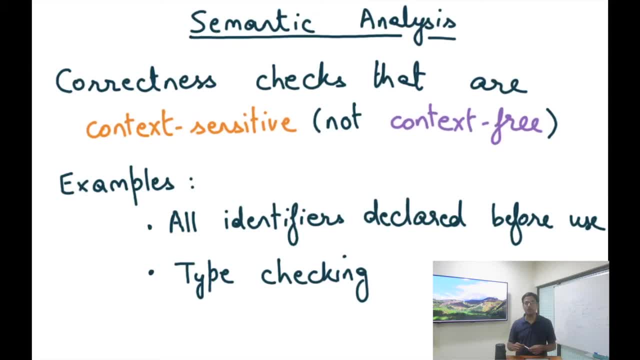 something is an identifier or not, which would be a, which would be an analysis of the lexer. but it's also about whether, what are all the identifiers that have been defined till this point. So that forms the context of of the program at any program point, and so you know whether the answer is yes or. 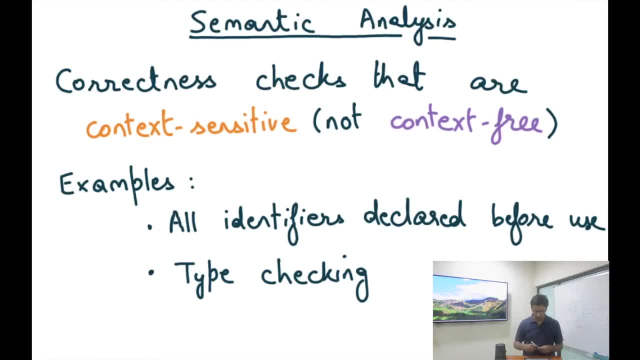 no, depends on what is the context at that point. for example, the context could be: what are all the identifiers declared until now? Similarly, type checking is a context sensitive analysis, as we're going to see soon. So the set of legal programs is a subset of the set of parsable programs. this 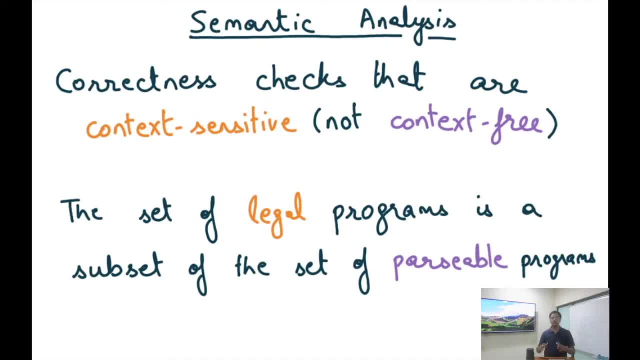 is generally true. we said that you know, some programs pass the lexing statement and some programs pass the parsing stage, and then all the programs that passed past the parsing stage are parsable programs. and then, and then the semantic analysis check stage is going to do some further checks on. 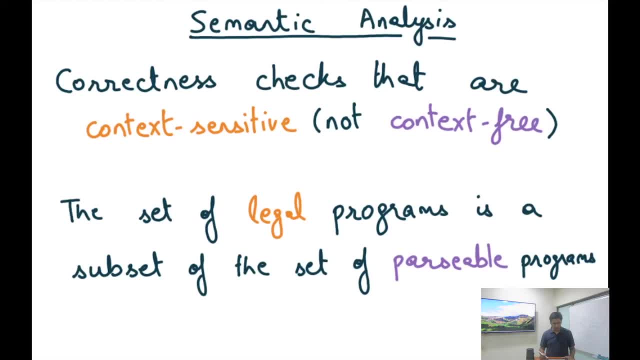 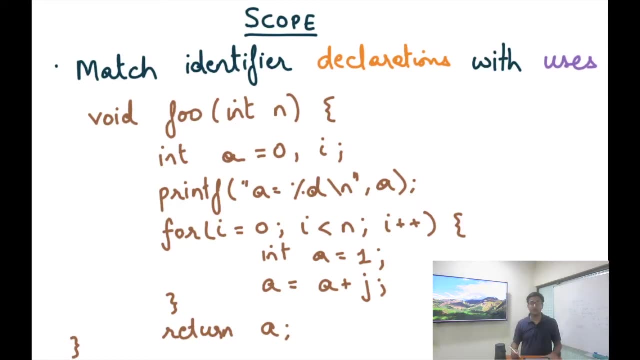 it and it's going to determine the set of legal programs, and these legal programs will be, you know, by definition, a subset of all the parsable programs. So here is an example of a semantic analysis of a set of legal programs. Context sensitive and semantic analysis is actually a very common analysis, which is scope. 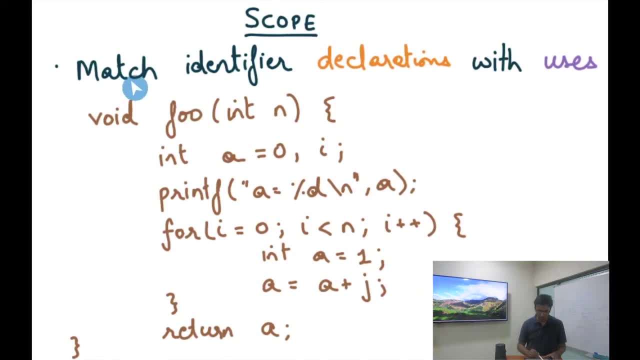 All right. so, for example, what is scope? well, you know we need. for example, we scope can be used to match identifier declarations with its users. So let's take this example program or example function from the C programming language, the function foo, that takes one argument, n, of type integer. 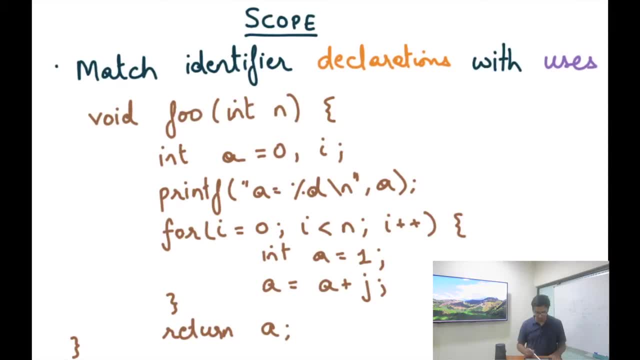 and it has some body. it's just an arbitrary body, but it declares some variables. so, for example, it declares a variable a and it declares another variable, i, and then it starts using some of these variables. for example, in this printf statement it's using the variable a. now what is a referring to? 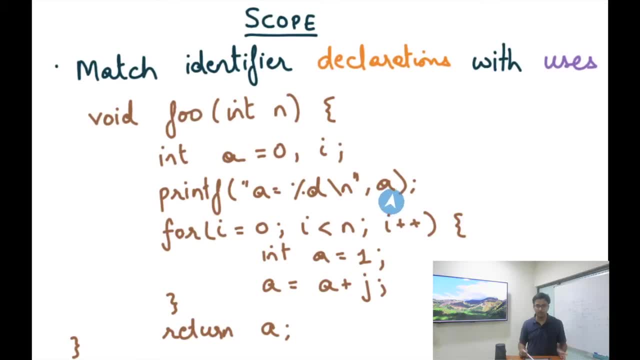 is determined needs to be determined because you know, a is just an identifier and the parsing state just said that a is an identifier and that's it right, and it just said that this is a function and it just said that it is also an identifier, but we never basically checked whether printf is. 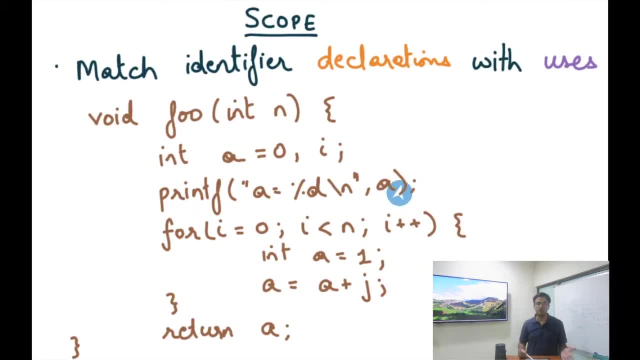 actually a function or not. we never really checked whether a is actually a defined, declared variable or not. These kind of things are in the come under the purview of scope, which is a semantic analysis. Similarly, here is a statement: for: i is equal to zero, e less than n, i++. given that the program 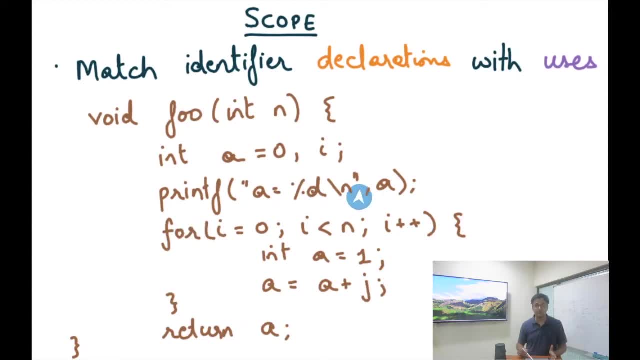 has reached the semantic analysis stage, we are already sure that this particular statement is a function defi rk. I, as less than n is less than i plus plus. given that the program has reached the semantic analysis stage, we are already sure that this particular statement is a function defi rk. 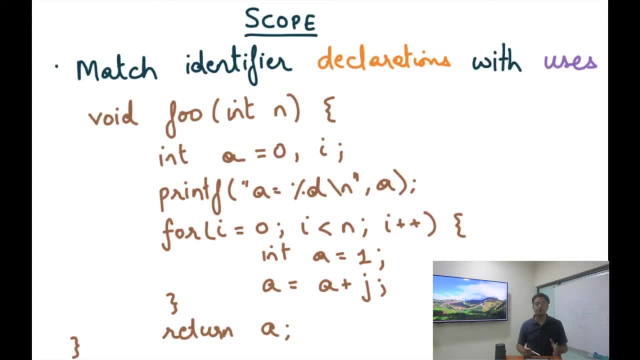 well parsable. What that means is that the for statement, the for keyword or the for construct is correctly formed. It has an initialization condition, it has a check condition and a step condition, and these are all the checks that are done during the parsing step, because these are 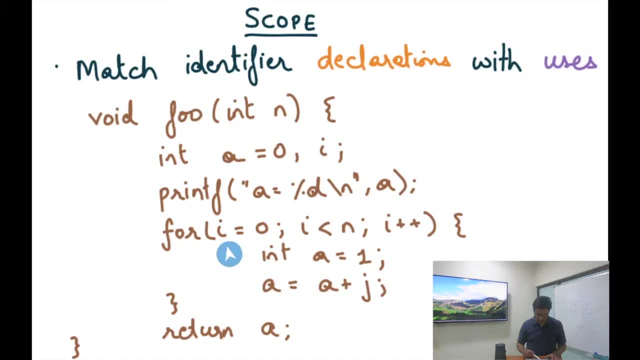 context free checks, But here are some context sensitive checks in the same example. Example: what is i? What does it refer to? That would be a part of scope, and in this case, this i refers to this one. Also notice that in this example, the body of the for function declares an other a. 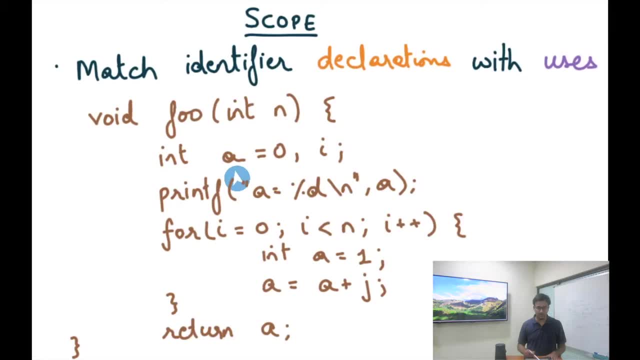 and this a is different from the a in the outside scope, and this a refers to the closest a that has been declared, and so on. And finally, when I come out of the for loop, I again use a, and this time the a is actually the outer scope a. So let us look at this. 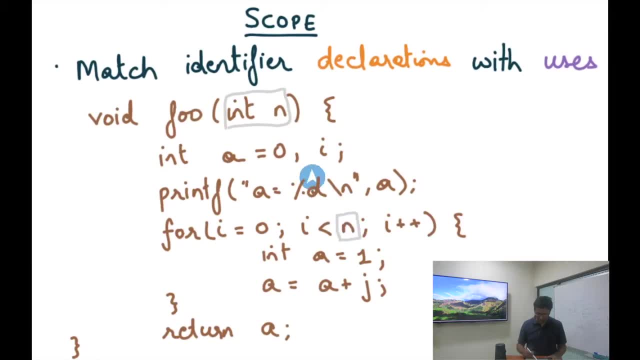 So, for example, what is n? Well, n is actually referring to this declaration that is coming from the function argument n. What are these two a's? These are coming from the outer declaration of int. a equals 0 in the body of foo. What is printf? Well, actually in this. 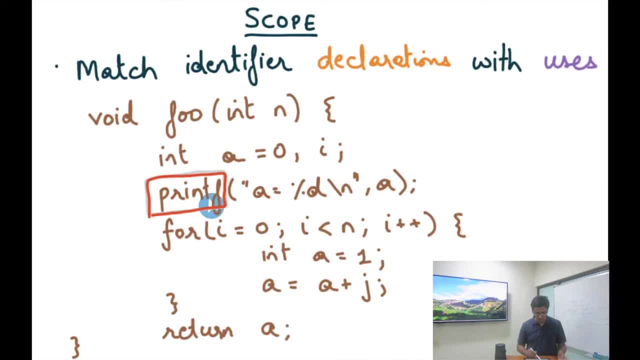 program fragment. I have not really declared printf. So you know, strictly speaking this is an illegal program just because of this. But if I wanted to, I could have declared printf printf somewhere outside of this scope of foo and then this would refer to that particular. 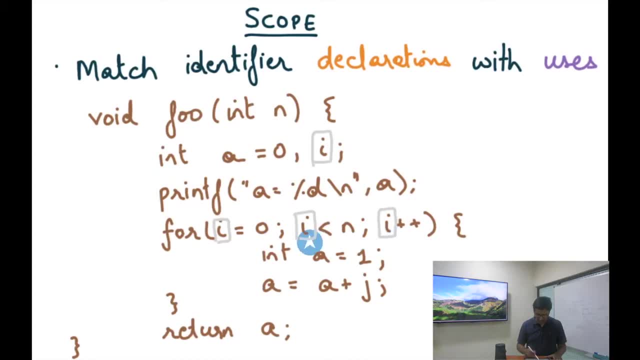 printf. What is i? Well, i is referring to this particular declaration. i and what is the a inside the loop body? Well, these two a's are referring to this particular declaration, that is, within the loop body. Okay, so these kind of resolutions of what does an identifier actually refer to comes. 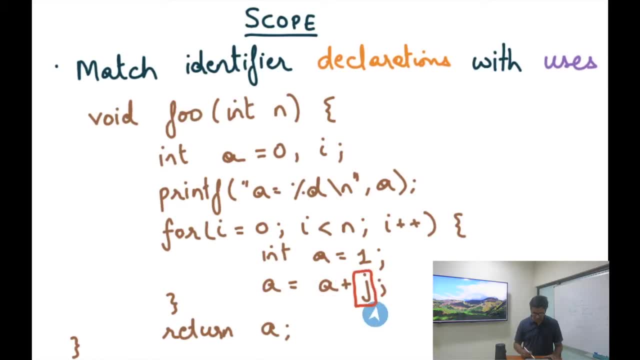 under the purview of scope rules. Also, here is another example: j, and in fact, if you see, j is not declared anywhere, and so this program has another error. None of these errors- printf or j- would be caught by the context free grammar, but they will be caught by the semantic analysis phase. in particular, it will be caught by the scoping. 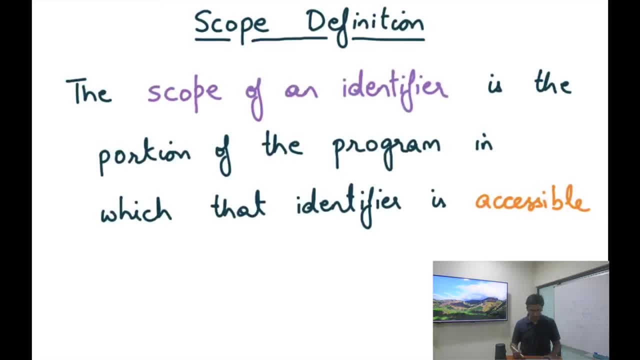 rules. All right. So what is the scope? Here is the definition of scope. The scope of an identifier is the portion of the program in which that identifier is accessible, All right. So, for example, what is the portion of the program in which i is accessible? 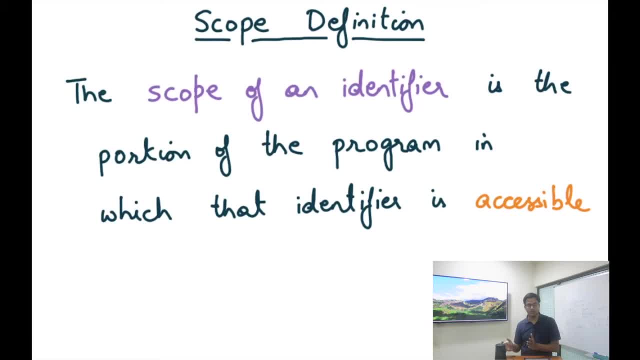 Well, it would be the entire function body after the declaration of i. Similarly, what is the portion of the program in which the second a is accessible? that would be the body of the identifier. Okay, So we would call this the form after the declaration of A, and so on. 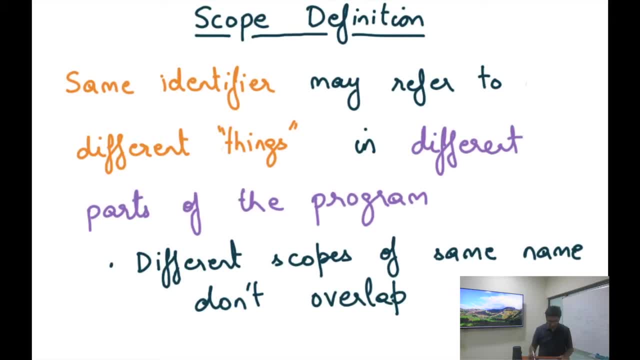 All Right. So some some subtleties about scope, which we may be already familiar with: Same identifier may refer to different things in different parts of the program. I am putting things in quotes and I am going to explain why, but the point is that the same 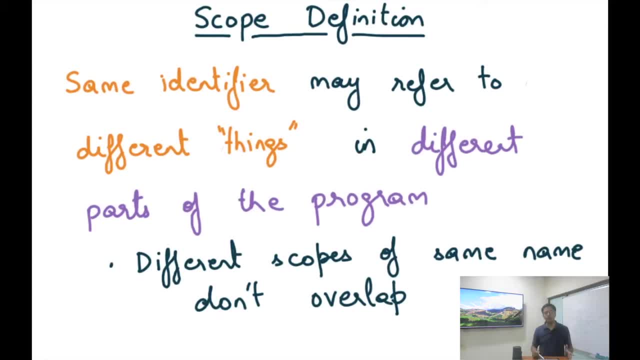 identifier may refer to different things in different parts of the program, And we already saw that with the example, The same identifier, A, is referring to different things. Okay, In one case A is referring to the outer declaration and the other case, A is referring to the inner. 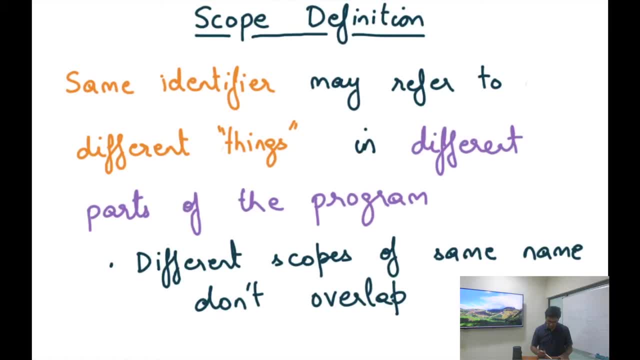 declaration of the for loop inside the for loop. So a corollary of this is that different scopes of the same name don't overlap. So, because we need a way to distinguish between identifiers, if the identifier has the same name, there is actually no way to distinguish. 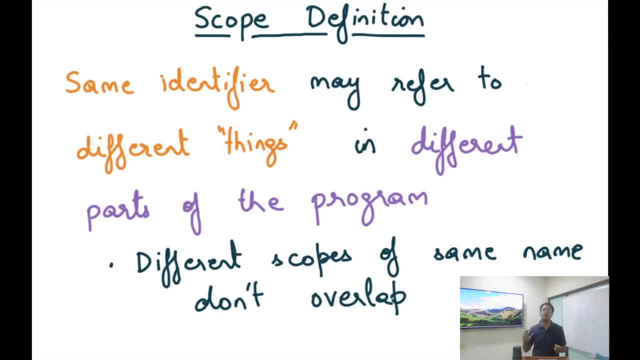 So if two different identifiers have the same name but they are actually referring to different things, then their scopes must be distinct. it can't happen that in the same scope both the things which have the same identifier name are present are accessible. Either one of them is so. for example, in the inner for loop, only the inner A is accessible. 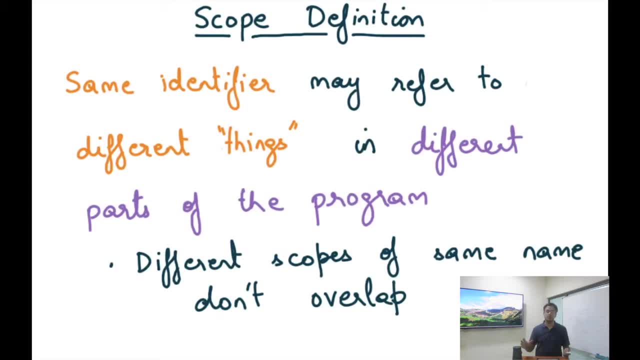 the outer A is not accessible, So the inner for loop is not the scope, Right, So the scope does not include that part of the program which is the inner for loop. after the declaration of the inner A: Alright, why do I say things and why do I put it in quotes? 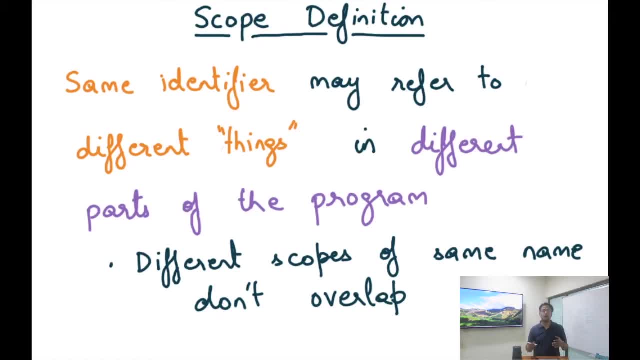 Well, because identifiers are used to denote or represent multiple things, They can be used to represent objects, memory objects. by objects, typically, I mean regions of memory, Alright, So, for example, a variable is an object. So when I say int v. 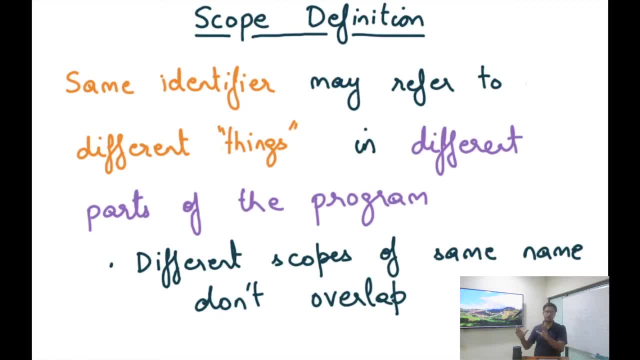 So I am basically allocating a region of memory for this variable v, And v is the identifier that denotes the object represented by v. But there can be other things that identifiers represent. For example, identifiers can represent types. For example, an identifier could represent a struct type in C, So I can say struct foo. 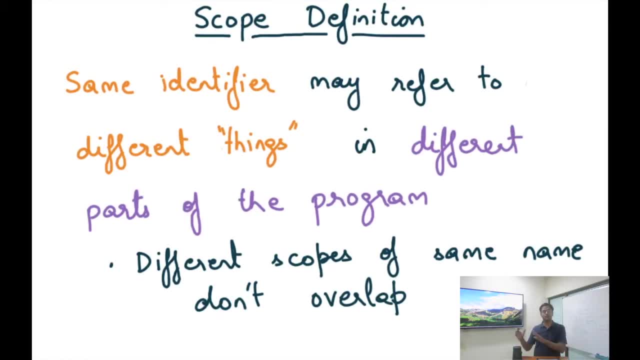 and something, And then whenever I say foo, struct, foo, then the foo basically represents that particular type that has been defined, And so that would also be qualified as a thing. It could be a function declaration. In object oriented languages, it could be a class name. 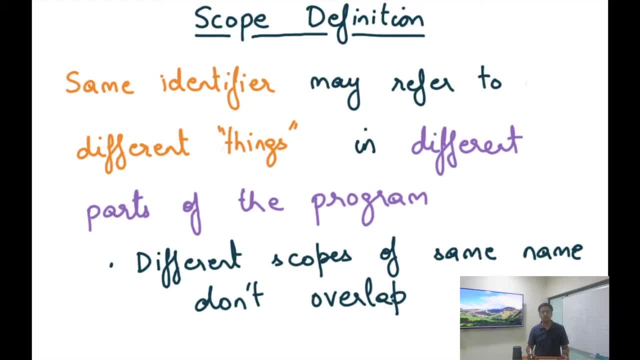 And there are other things that you could do with identifier names, For example, template names or template type variables in languages like C++, and so on. So identifiers are used to represent different things and everything should have some type of scope rules. So it is saying that what identifier can represent what thing at what point, based on the structure. 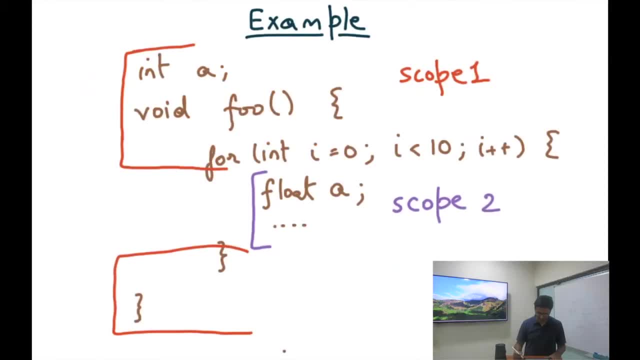 of the program as defined by the scoping rules. So in our example we said that there are two objects in this case. One is A and the other is another A, And this time to distinguish it I just use float different type for the second one and the first one is still an int A, And notice that the scope 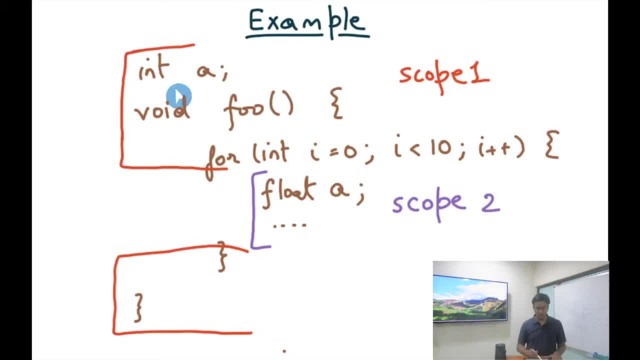 1. So I am using scope 1 for the scope of the first A, The integer A, and that is represented by these red lines. The notice that it does not include scope 2, which is the region where the second A, float A, is accessible. 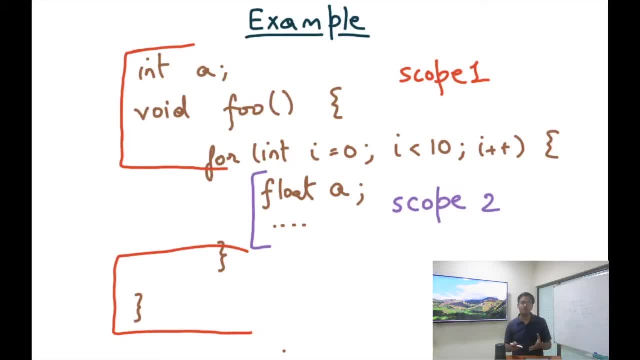 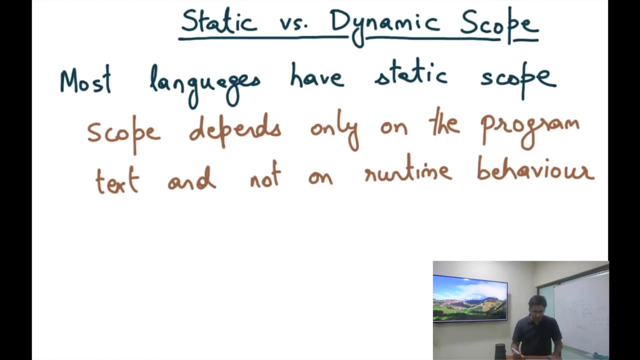 So scopes of different objects can overlap, But if the two objects have the same name then they cannot overlap, Because if they overlap then there will be an ambiguity. Okay, So there is another. scope is of two types, typically in languages. One is static scope and other is dynamic scope. 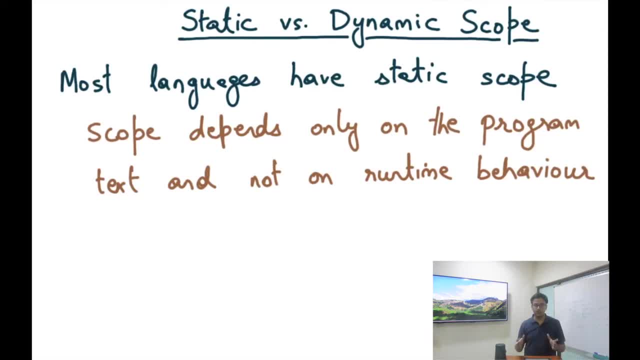 Most languages use static scope, and that is why most of us are familiar with static scoping. In fact, the example that I used was using static scoping. More formally, if the scope depends only on the program text and not on runtime behavior, then it is called static scoping. 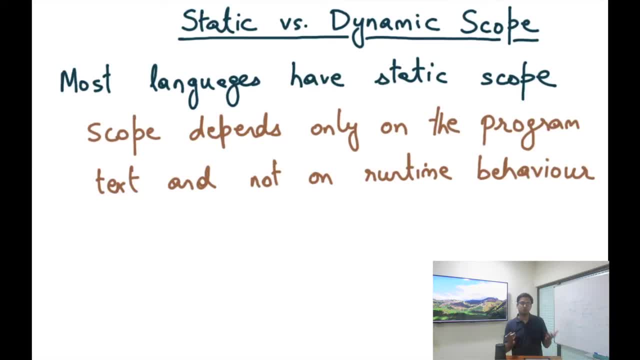 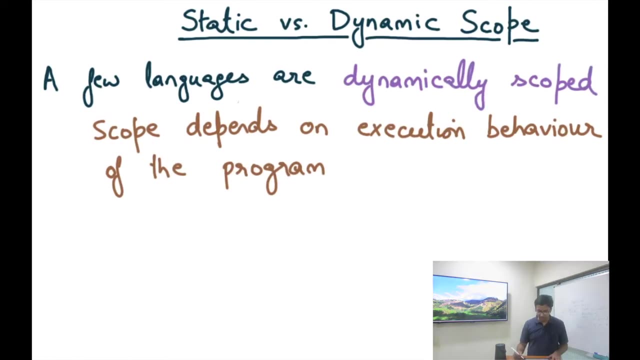 Alright. So, in fact, all the examples that we saw. where is A accessible? it only depends on how the program is structured and has nothing to do with the runtime behavior of the program. In contrast, a language could be dynamically scoped. In this case, scope depends on execution behavior of the program. 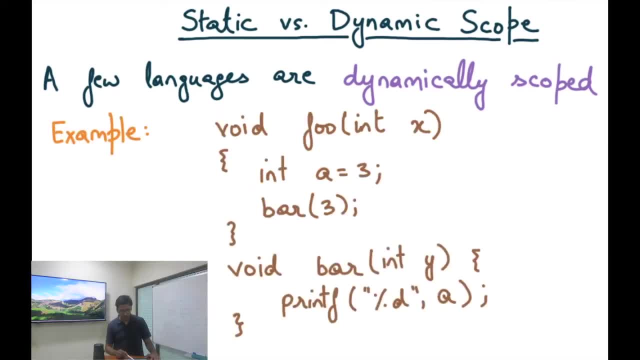 So let us take an example. let us look at this example, which has two functions, and let us assume that this is a dynamically scoped language, although I am using C-like syntax, but C is not statically scoped, while this language I am assuming to be dynamically scoped. 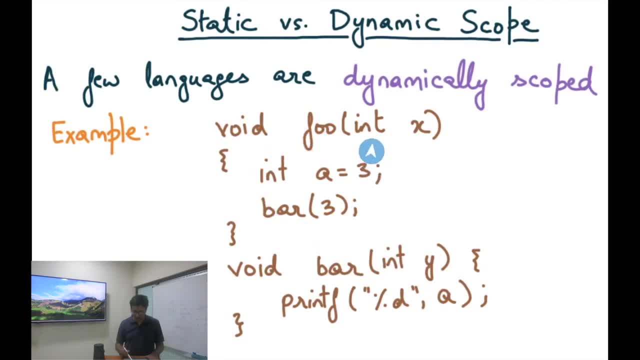 And let us say: you know, in a dynamically scoped language, let us say I define a function foo and then I call bar from the function after declaring a variable A. Now inside, in a dynamically scoped language, what could happen is that inside bar I could actually access A because A seems A is in the 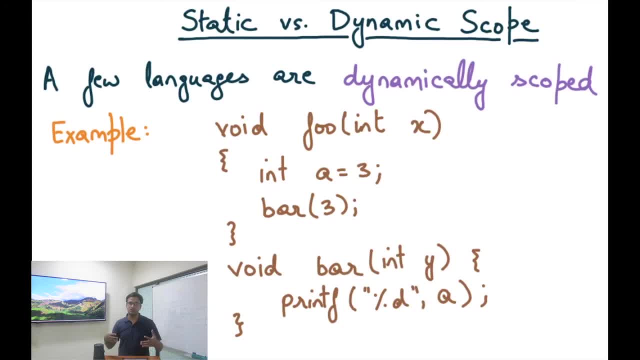 Okay, Run time: set of mappings for this particular program, right? So, for example, when I call bar 3 and I say printf %dA, then I can expect if it, if this is a dynamically scoped language, then I could expect that this is going to print 3, because 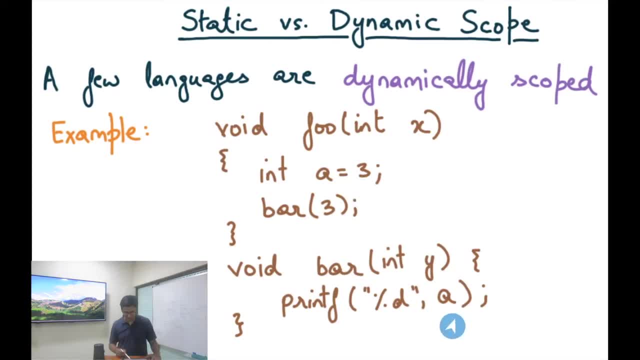 of the declaration, A equals 3 here. Alright, So this is. this would be a dynamically scoped language. Notice that A is not present. It is present in the static scope of the language, but A is present if bar is. A is present in the dynamic scope if it has been called from foo. 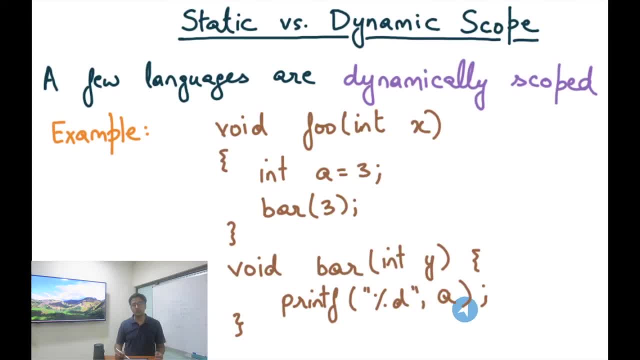 You may ask what happens if bar is called from from a function where A is not present. For example, let us say we have a function called foo2 or bars, which basically calls bar without declaring A. In that case that would be a runtime error. 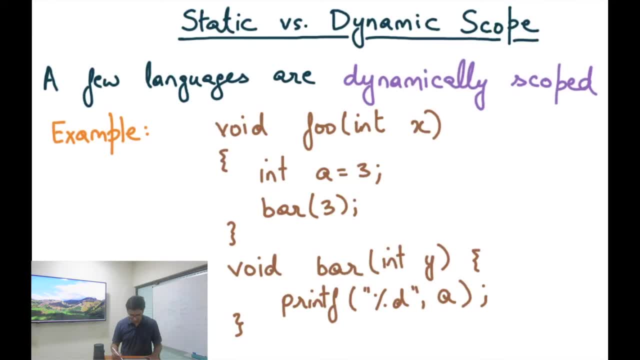 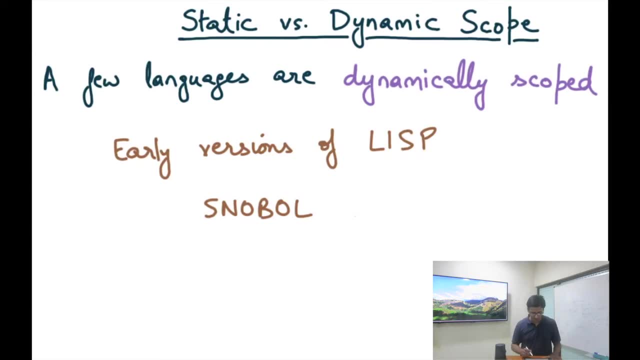 Alright, So that's. those are the kind of semantics that some languages would have. What are some language examples of languages that used dynamically scoping? first of all, it's extremely rare today, but there were early versions of Lisp that used dynamic scoping before Lisp actually transitioned to static scoping. also, 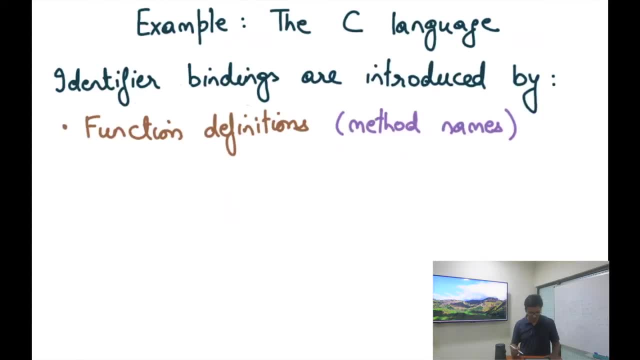 there's a language called Snowball that was using dynamic scoping. Alright, so let's take an example to understand. how do identifiers get declared and then what are their scope rules? so identifier bindings are introduced in different ways, in different languages, in fact, and also we said that identifier bindings could bind to different types of things, right? so 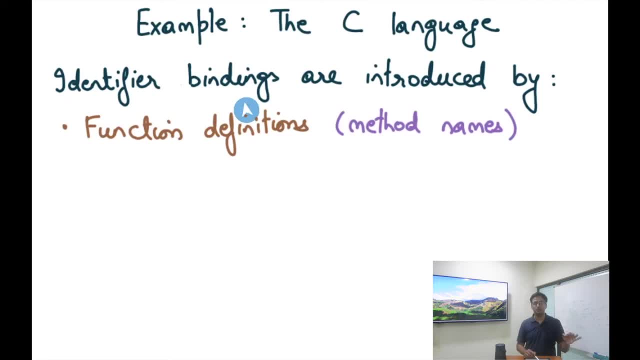 they could bind either to objects or types or function declarations or something else, right? so identifier bindings are introduced by different things, so, for example, they could be introduced by function definitions. i could define a function called, let's say, printf or foo, and that would be. that would introduce a binding. every time a binding is introduced, we also need to basically 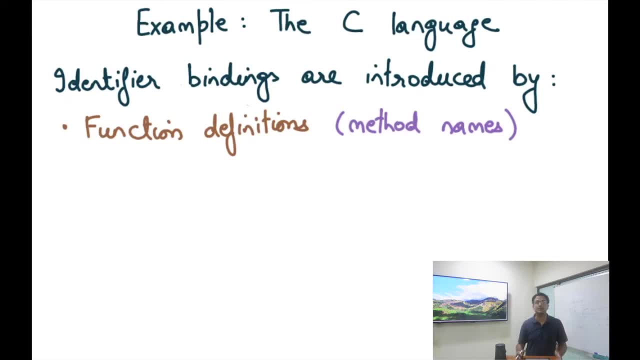 say: what have some rules to say, what are the scope under which that binding is accessible? all right, so function definitions are a way to introduce bindings for method methods and these bindings basically give you method names and so that way you are able to access those methods. similarly, strep definitions in c provide bindings for type names. variable definitions provide: 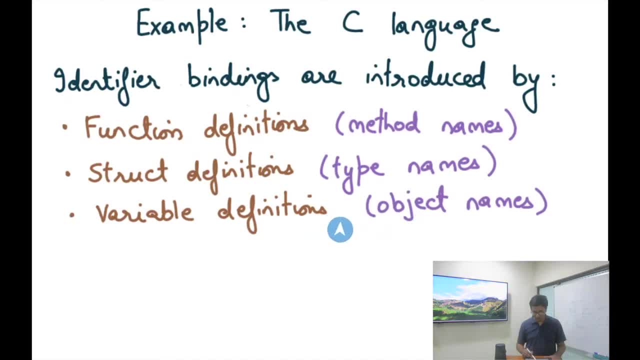 access, introduce object names right, so they provide bindings for names to objects or recall that objects are nothing but regions of memory structure field definitions. so inside, inside of a c struct, i could say int a, int b. these would be the fields of that particular struct and they are also basically 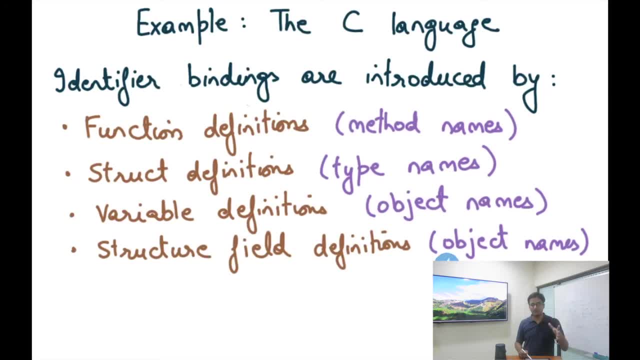 names, for you know, you can say sub objects of objects of that particular type, and so i'm also using the words書 and k to for conditions as well. you can say sub objects or object names, although they are kind of sub objects of a type s o. that's where they are different. 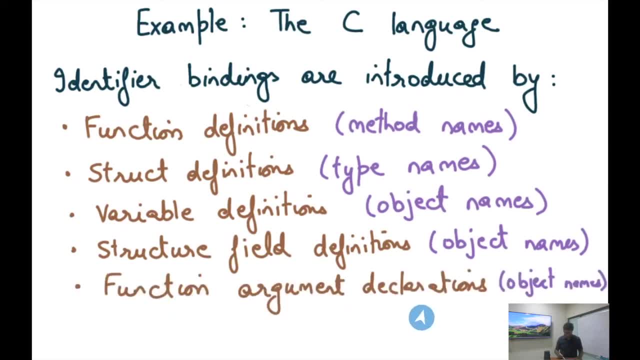 type of findings actually, and then function argument declarations, so i can also create bindings because of function argument declarations. we saw that in our example. for example, if the argument is int n, then i have created a binding from n to the argument value and depending on whether it's a call by value or a call by reference, 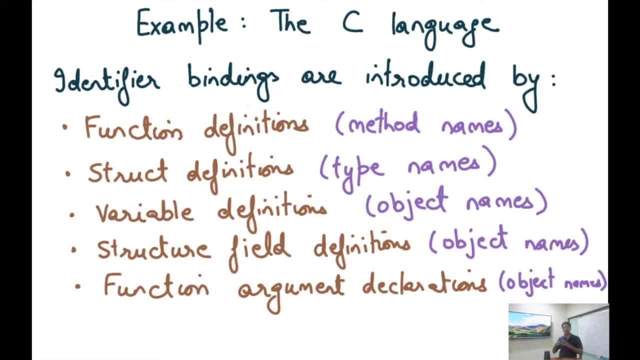 it's either a temporary copy of the argument or you can substitute it in that way of binding. it's like just suppose you want to carriage it. the roExploit technique percentage. and then, if this happens, why did i die? when this happens, whether is i loading inaca精? so, in fact, even if you, if the argument on already inaca's written by 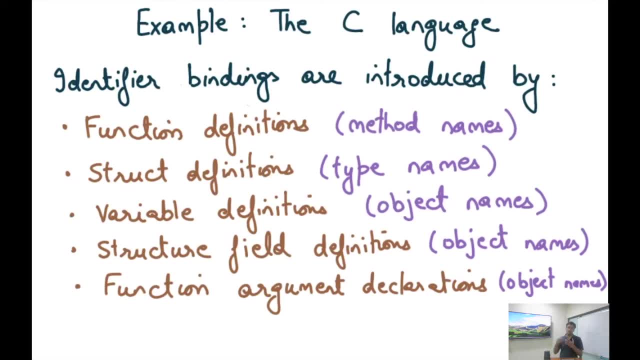 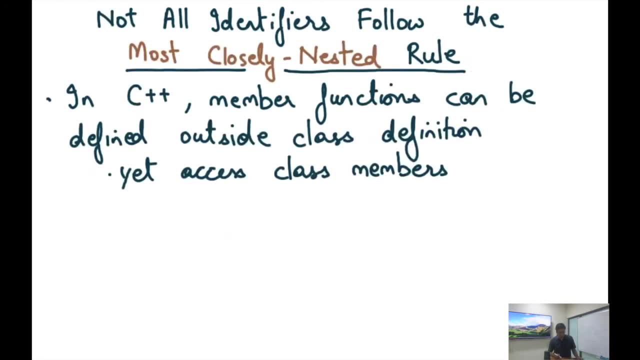 that was passed from the caller, or it is actually a reference to the, to the object, that that is existing in the caller. all right, okay, here's in some interesting facts about scoping. typically, scoping rules obey the most closely nested rule, which means that if I use an identifier a, then I basically 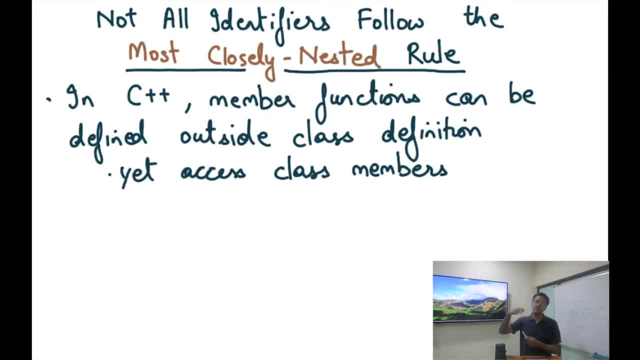 look at the most closely nested declaration of a. so we saw this example where if I use the a inside the body of function of the for loop, then that particular use is basically binding to the closest declaration, the closest nested scope in which it was declared. in this case it is the scope of the for. 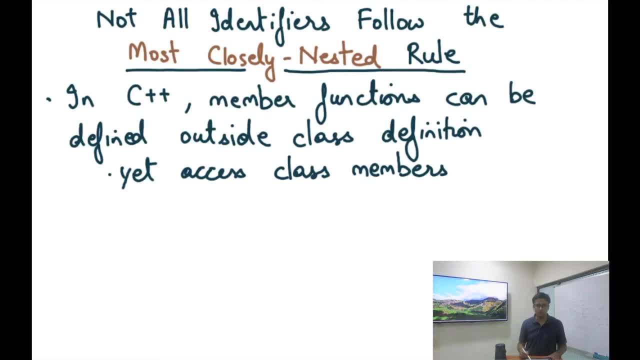 loops body. so that's called the most closely nested rule. okay, and many most scoping rules basically follow this rule. however, there are exceptions. for example, in C++, member functions can be defined outside class definition and yet access class members. so in C++ you could have a class definition and you could have members of the class, and then you 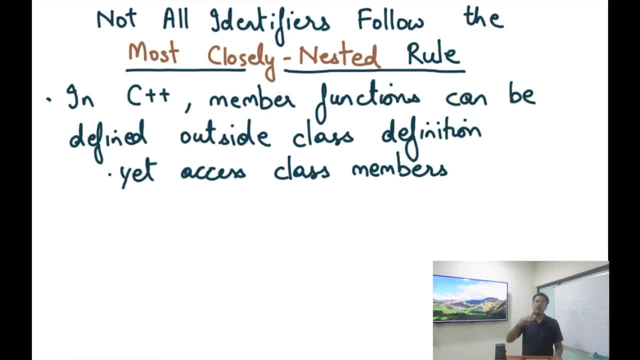 could have some methods or functions inside the class member functions and that the definition of that function can appear outside of the class. also, these, the body of these member functions, can access the member objects of the class from within the body. now notice that in the static scoping nesting rule that we have just observed, the function that's defined 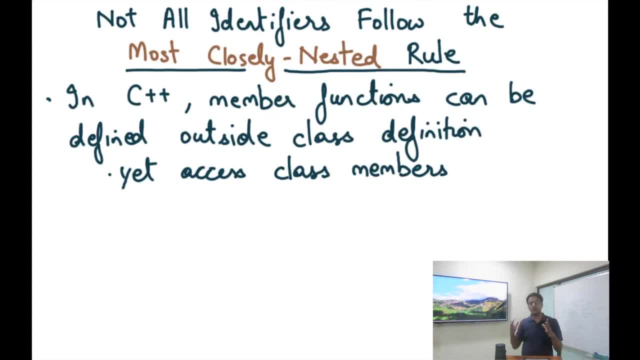 outside of the class does not actually have the member variables declared in any of the nested statics, statically nested loop scopes of that definition. but but still we are able to access it and that's because the, the rules, basically permit a you to also access the class and, and that's given by the, the qualification of 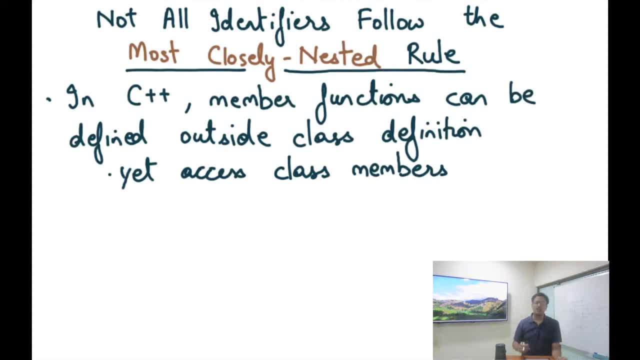 the member function definition using the class name and things like that. you know, those rules are also pretty easy to understand, just that they're not following the most closely nested rule and this is an exception to that that rule. actually there are more exceptions, for example forward declaration. so 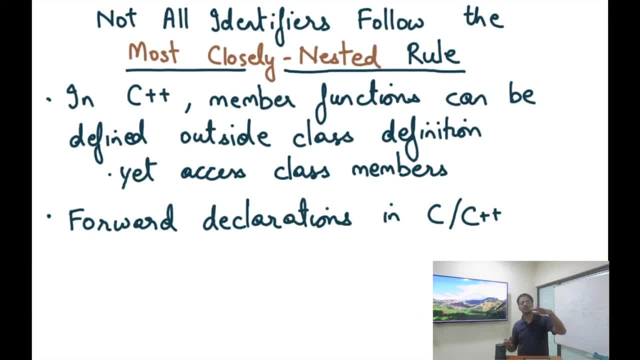 typically we would imagine that something should be used only after it has been defined, right or with the declaration and the definition. but often there are forward declarations in CNC plus plus where I could define something using an external keyword and then actually actually declare you something with an external keyword and then define it later and use it in the 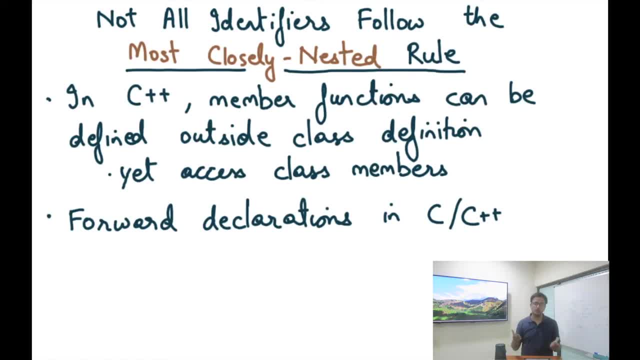 middle. so so those will be called forward declarations and they would also. there also exceptions to this rule, that thing. you just just look upwards for the and look at the closed closest nested rule, scope- most closely nested scope- to basically identify the object or the thing, whatever you're looking for. there are also examples in C++ where you know. 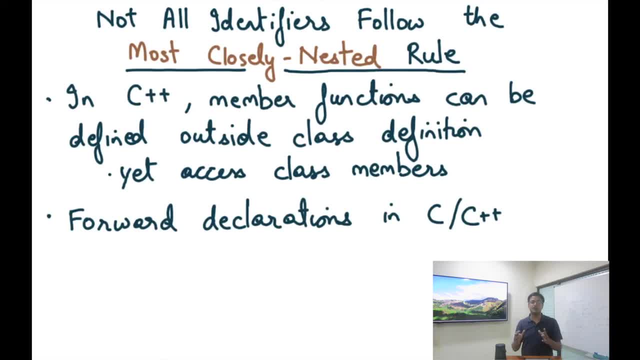 you, for example, in: within a class in C++ the member objects can be defined later but accessed earlier in the function bodies, and that's perfectly okay, in which case the order is really immaterial whether I define, as long as those member objects are present somewhere in the class declaration, we are okay. and